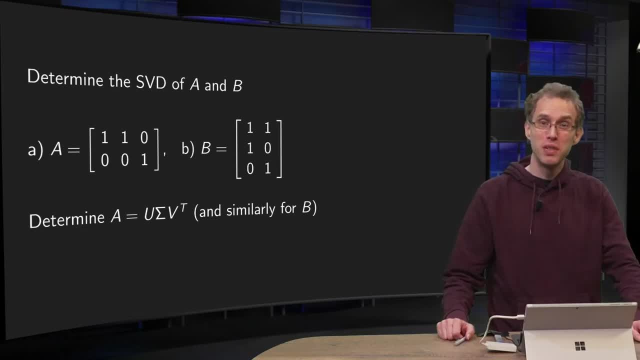 We have already seen the procedure to compute a singular value decomposition of a matrix. Let us now look into two explicit examples to see where the technical difficulties arise in some specific cases. So we have a 2x3 matrix A and a 3x2 matrix B and we are going to compute. 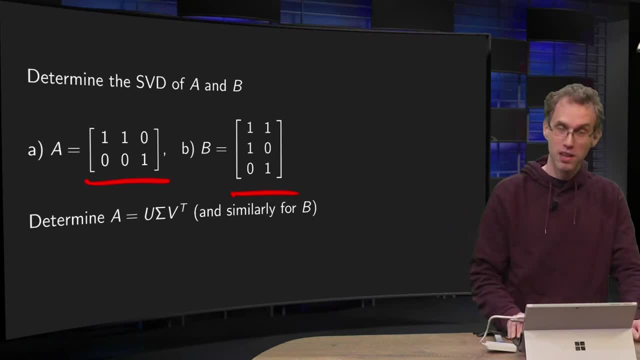 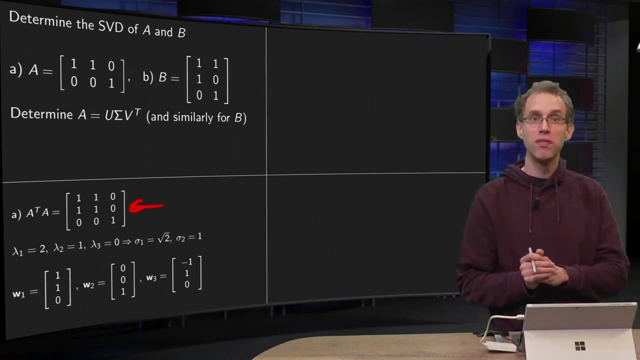 the singular value decomposition of A and of B. Let's start with A. So what do we need to do To compute A transpose times A? well, you can do that yourself. and then you need the eigenvalues of A transpose times A. Well, you already see the 1 sitting here, so 1 will be an eigenvalue. 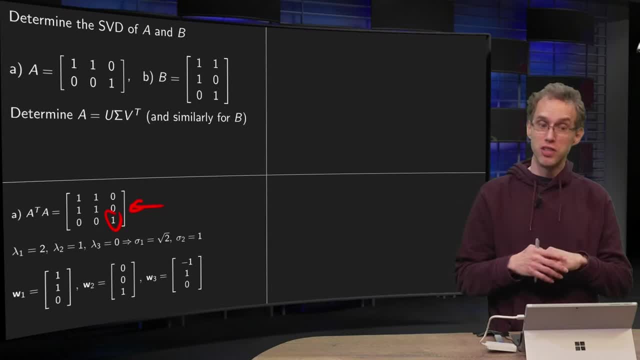 You see, two rows are the same, so the matrix will have a zero eigenvalues. so you know 1 and 0 are eigenvalues, and then you can use a trace to compute the third, which is 2.. So eigenvalues are 2, 1 and 0.. 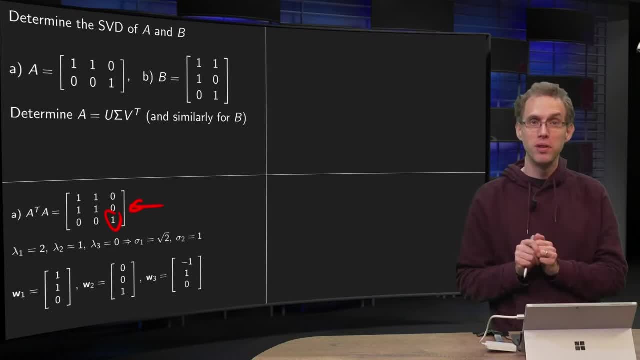 If you want, you can use the characteristic equation as well, of course, but this is a bit far. So then the singular values will be the square root of 2 and 1 and 0, but we are not going to use that one, Only the square root of 2 and 1, we only 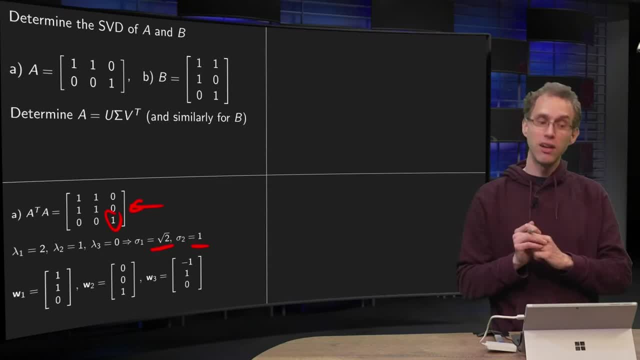 use the non-zero singular values, Then you have to compute all the eigenvectors. so if you just compute eigenvectors without bothering about norms or whatever, you will get 1, 1, 0, 0, 0, 1 and minus 1, 1, 0 for our three eigenvalues. 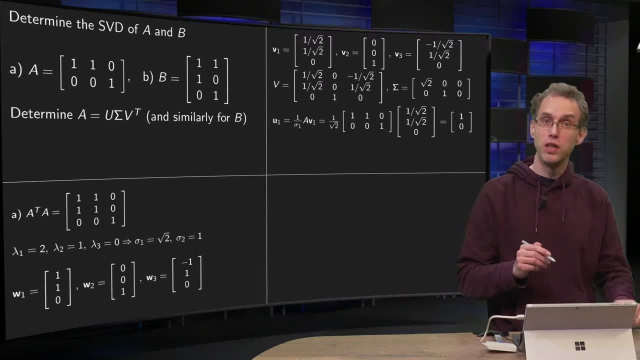 Then we can compute our singular values. So if we compute our matrix V first, we normalize our eigenvectors. so V1 has to be normalized, W2 was already normalized, and W3 has to be normalized, and there you have your V. 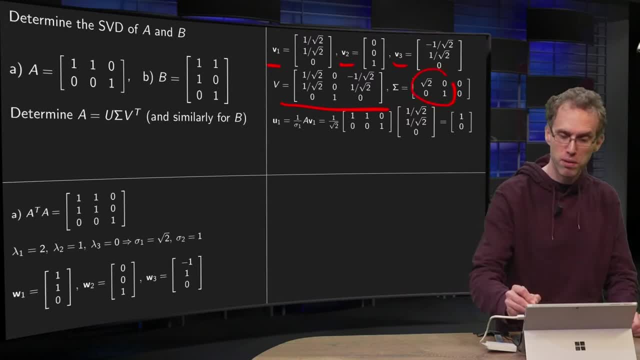 Then we can form the diagonal block of our sigma. put the singular values, you need to get a 2 by 3 matrix, so you have to add a column of zeros. so there, you have already your sigma. Now we want to compute our sigma. 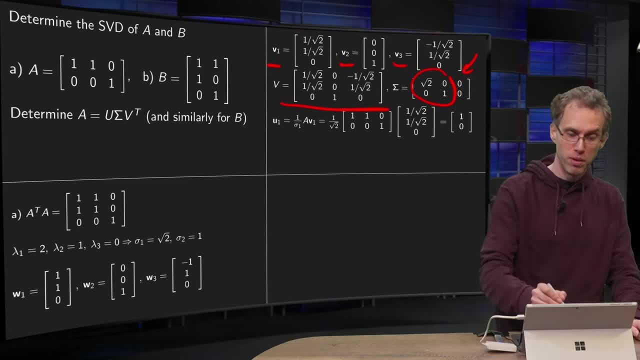 Now we want to compute our sigma, Now we want to compute our U1.. So your U1 will be 1 over sigma1 times A times V1.. So here you have your 1 over sigma1, here you have your A and here you have your V1. 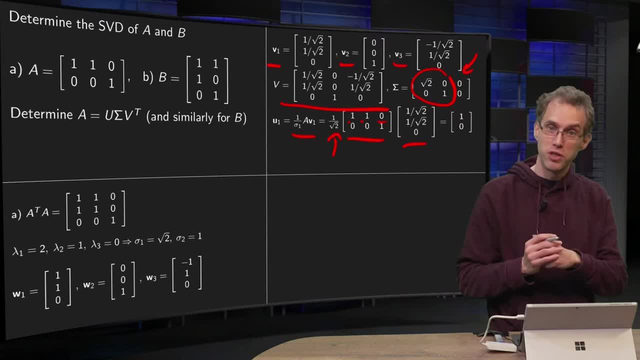 So, for example row-column rule, you get 1 over square root of 2 plus 1 over square root of 2 plus 0, so 2 over square root of 2 divided by square root of 2, gives you a 1, and your 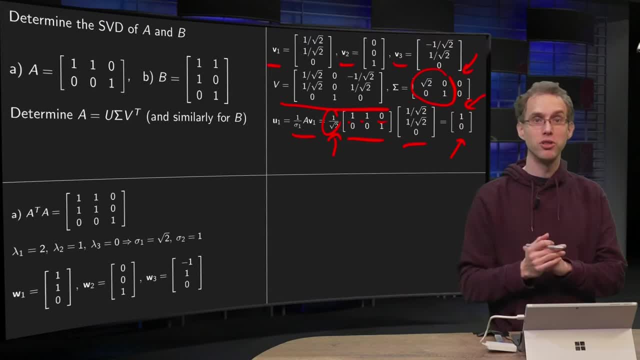 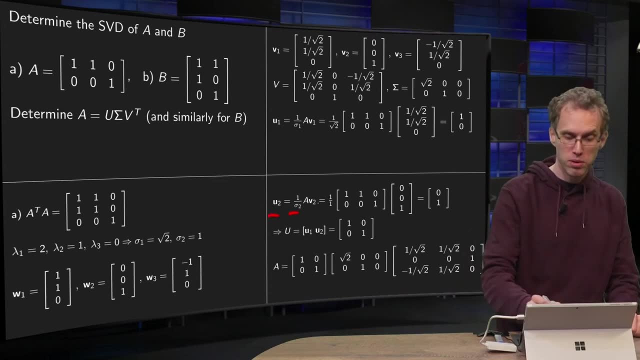 component- you can do it yourself- gives a 0. So U1 will be 1, 0.. automatically normalized. Similarly, you can compute u2, you have 1 over sigma 2 times a times v2, sigma 2 equals 1, so you get a 1 over 1, here you have your a and here you have your v2,. 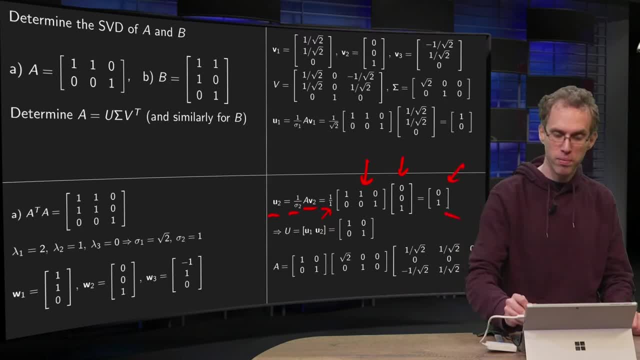 so the first inner product is equal to 0,. second inner product to 1, divided by 1, so you get just 0, 1, so there you have your matrix U and there you have your singular value decomposition for the matrix A. 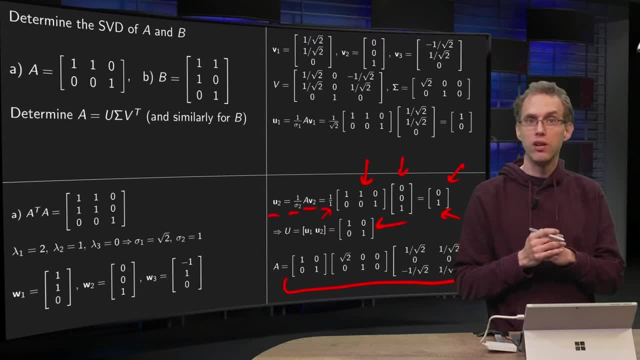 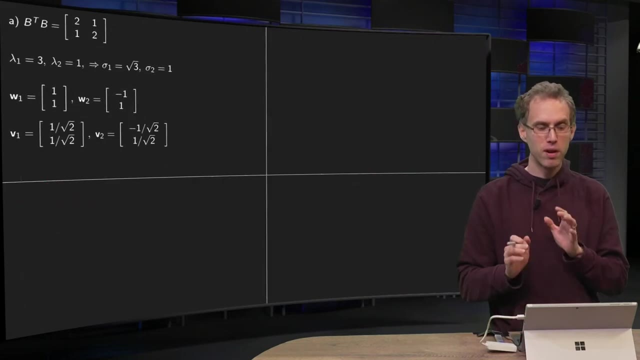 So, as you see, not too difficult. very similar to the computation of a diagonalization of matrix A. Let's move on to matrix B, because there is a slightly tricky part somewhere. as you will see, First part goes similarly. Compute your B. transpose times B to where 2,. 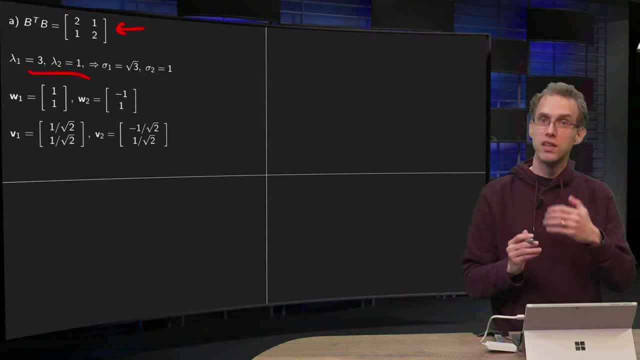 now your eigenvalues will be 3 and 1, as we did in an earlier video, so your singular values will be 3 and 1.. Squared of 3 and 1,. compute the eigenvectors first, without bothering about norms. 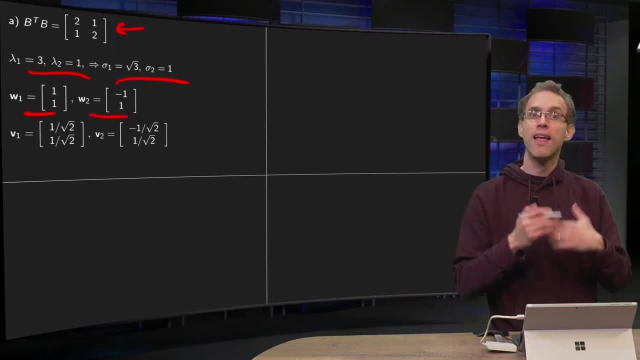 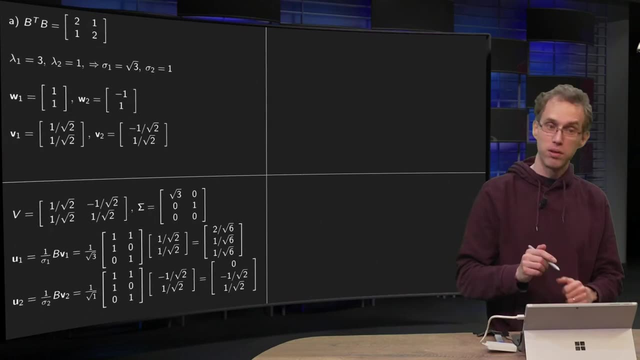 w1 equals 1,1 and w2 equals minus 1,1,. and then you need to normalize again to get your v1 and v2.. So far, so good. Now forming your v is easy. just put v1 and v2 in your matrix. 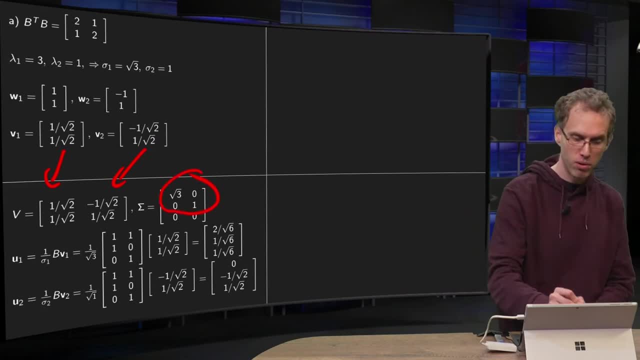 forming your sigma is easy: put the diagonal block and add, in this case, a row of zeros to get a 3 by 2 matrix. so there you have already your matrices, v and sigma. But now u, u1 is clear. compute: u1 equals 1 over sigma, 1 times B times v1,. 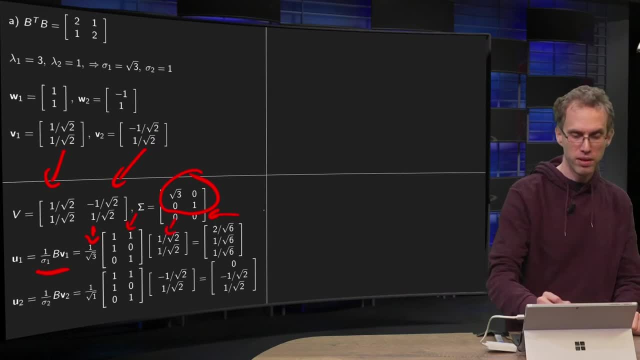 so here: 1 over sigma 1, the B and the v1, you can compute it yourself. there you go- and u2. similarly, 1 over sigma 2 B times v2,. 1 over sigma 2 B, v2,. 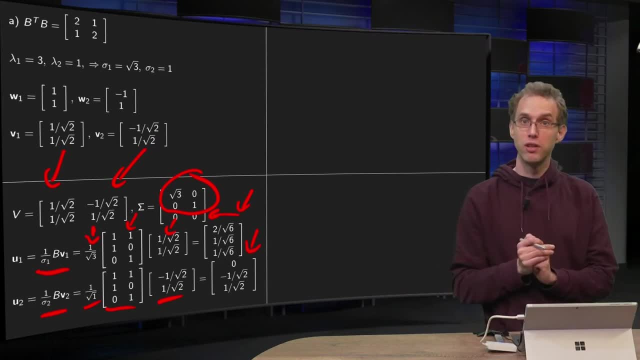 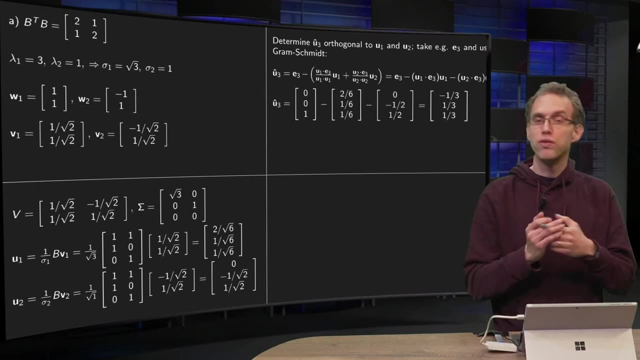 compute yourself. there you have your u2, nicely normalized and orthogonal. But now we have to determine some u, u3.. So first we determine the u3 hat, without bothering about its norm yet, which is orthogonal to u1 and u2.. 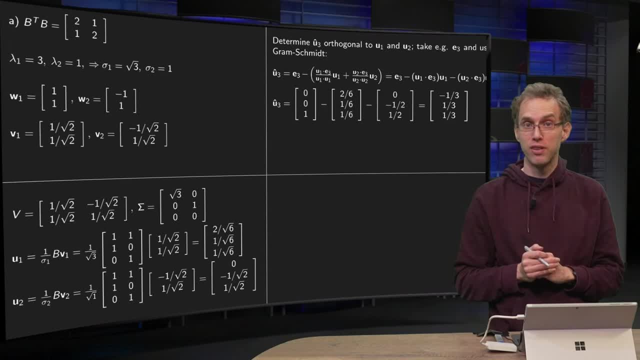 So we just take some vector in R3, hope it is not in the span of u1 and u2, hope it is some other vector like that. so just take something like 0,0,1, for example, an easy one. 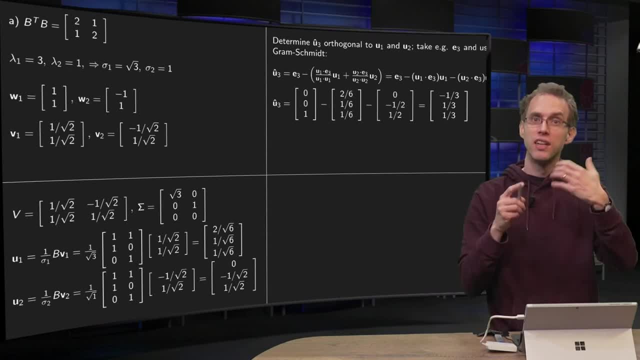 and then we use Gram-Schmidt to form an orthogonal basis and in that way we find our third vector for our matrix U. So we take, for example, e3,. you can take e1 or e2 or whatever your favorite vector. 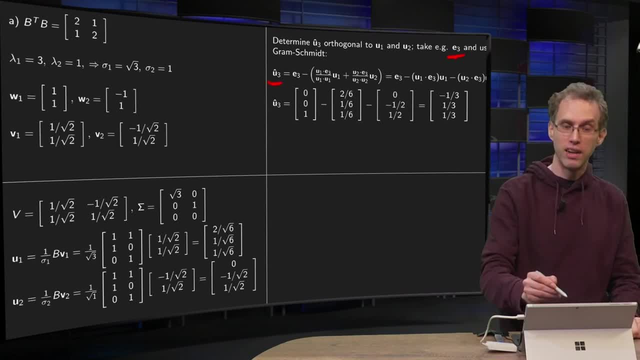 and then use Gram-Schmidt u3, hat will be then e3, minus its projection on u1 and u2.. Now what a nice part is that u1 and u2 are normalized, so the denominates are both 1, so the equation simplifies a bit until this expression: 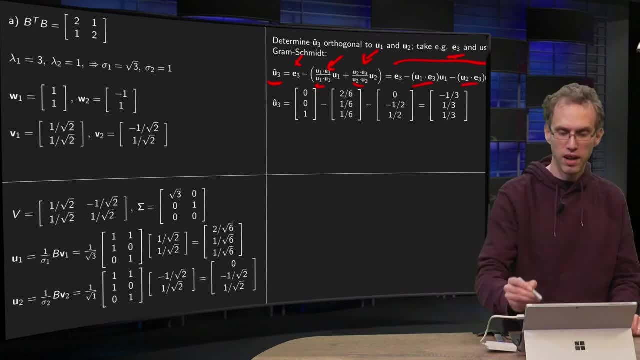 but you still have to compute those inner products here and there and you end up with your e3 minus the first vector, minus the second vector, and this gives you minus 1 over 3, 1 over 3, 1 over 3.. 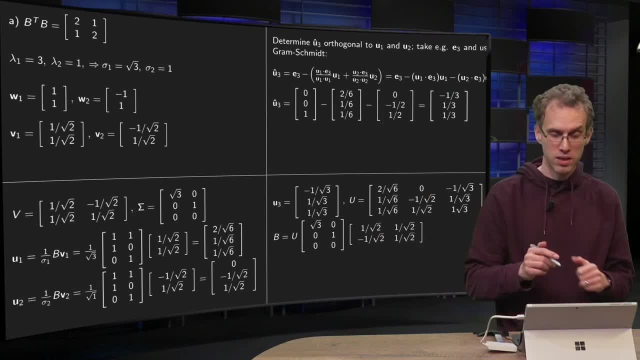 And of course you have to normalize that. so your u3, and if you normalize this vector over here first, you can for example turn it into minus 1, 1,, minus 1, 1, 1, and then normalize.